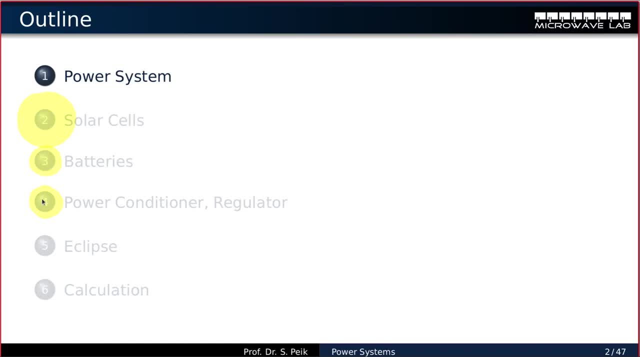 need some kind of power conditioning and regulation. At the end I will talk a little bit about the eclipse of a satellite, because this is the main driver of the stored battery power, and we conclude with some calculations and some examples of power subsystems. Well, the power subsystem has several. 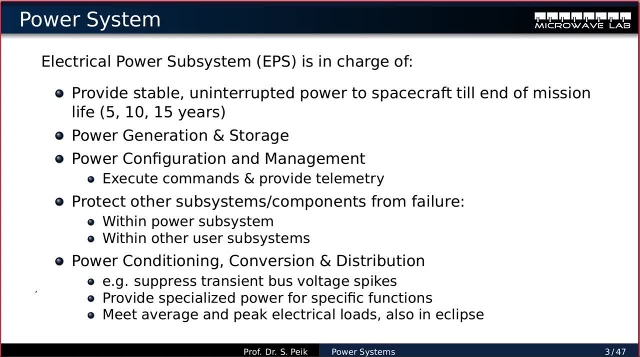 purposes. The first one, of course, is that it has to supply uninterrupted power to the satellite such that it can operate, and this is done by a generation of power and the storage of power, and it must configure the power with the certain levels of voltages and currents and so on, and then also it has a 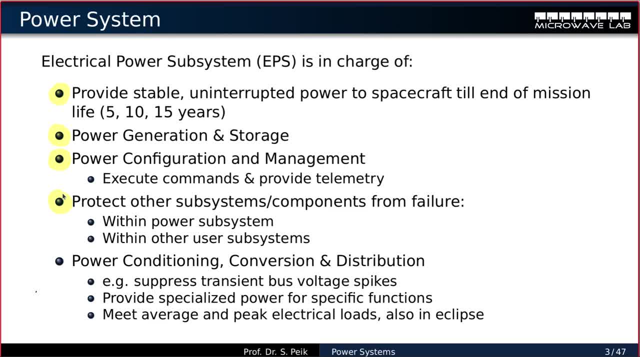 requirement that it protects other components from failure. for example, if one of the components has a short, then the satellite must shut down that component, and the satellite shall still operate and well. finally, it has to suppress transients, for example, and provide special power features and functions. 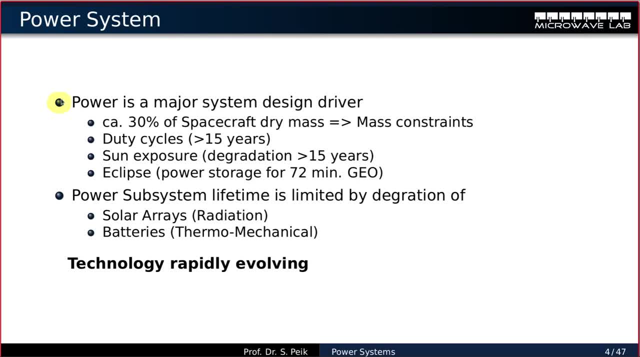 Well, as I said, the power baikd, The power subsystem, is a major system driver of the whole satellite. As you see here it makes up about 30% of the spacecraft mass, which is a considerable section of the spacecraft. That means you have to put a lot of attention into your power subsystem. 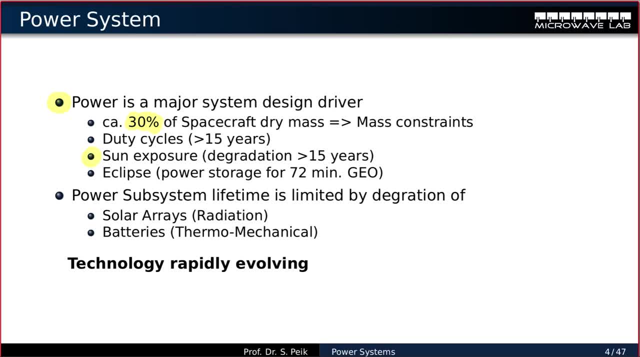 Please note that the solar cells are exposed to light and eclipse where the temperature of the satellite goes up and down. This is also a main limiting factor of the lifetime of a satellite, because the solar arrays degrade and the batteries degrade. That's why, besides running out of fuel, 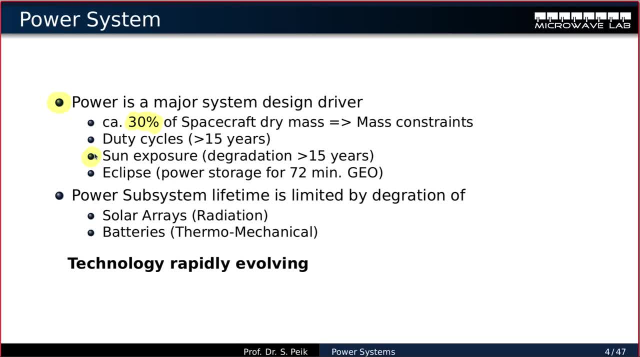 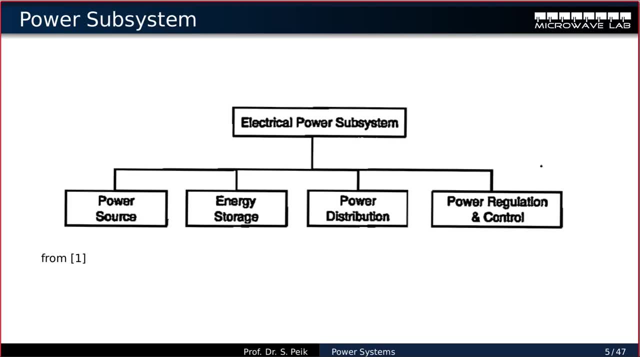 the satellite, life is limited by the power subsystem. due to these reasons, When we look at the subsystem, we have four major elements. We need a power source in our power subsystem, where the power comes from. Then we have to store energy for eclipse times and for energy peaks. 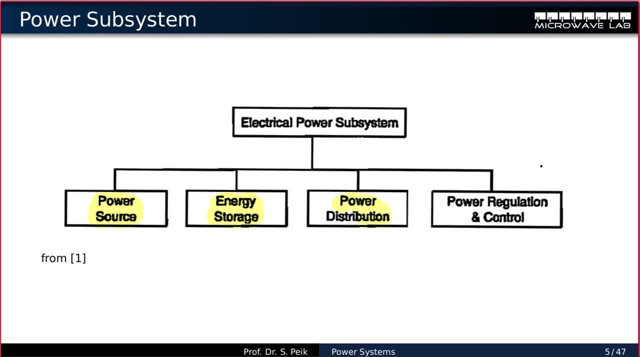 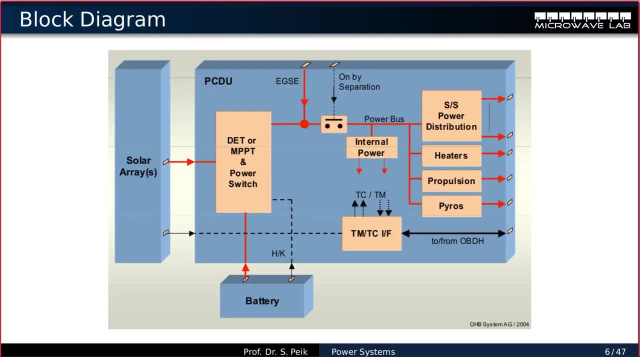 Then we need components to do the power distribution And we need components to do the regulation and the control of the power. I will go step by step through these four elements. now Here's a block diagram, courtesy of OHB, which shows the real system setup of a power subsystem. 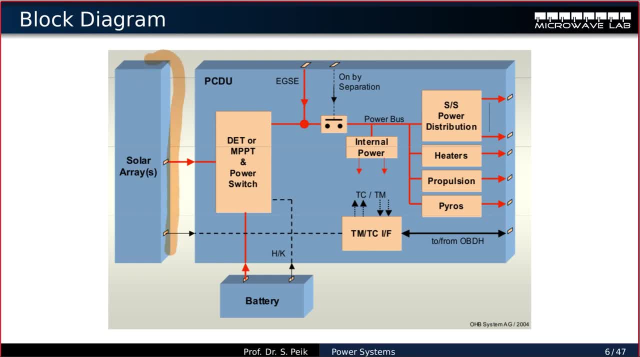 Here on the left side we have a solar array where the power is generated, And we also have a battery where the power can be stored, And in between we have a maximum power point tracker. I will explain this in a second. Let's see how this works. 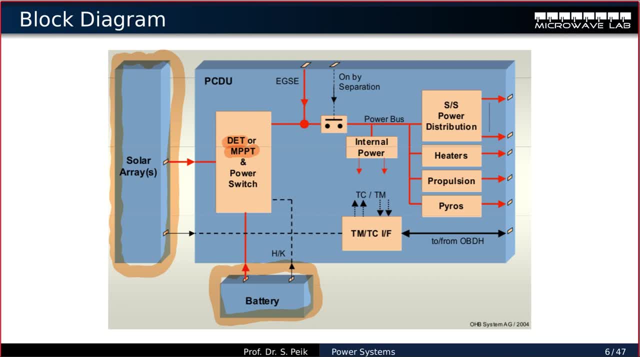 And switches, or a so-called direct energy transfer, which transfers my energy directly to the power bus. Usually there's a switch built in here. The switch is off until the satellite is launched, such that we do not drain the batteries and we do not power up the system while it's in assembly. 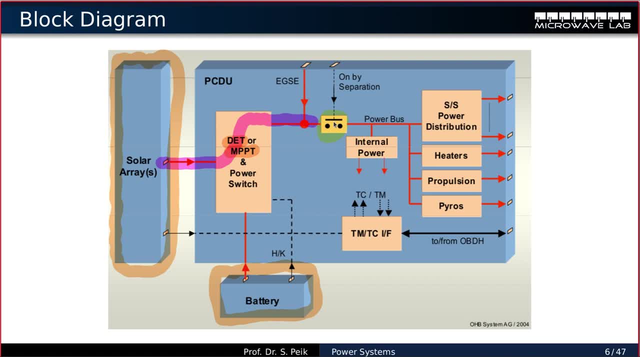 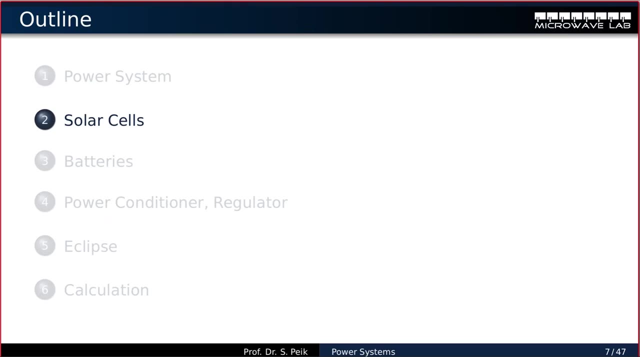 Once the satellite is separated from the rocket, it powers up by closing that switch And then it powers up all these elements of the satellite. Okay, first part, The solar cell. We can power up the satellite by various means. By far most popular is to power the satellite by solar cells. 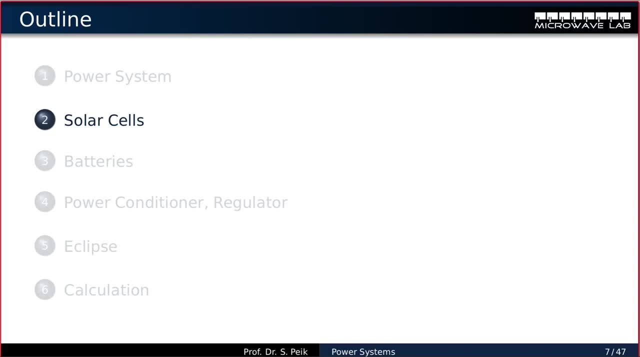 Alternatively, you can use nuclear power like so-called nuclear batteries or spring-loaded assemblies or some other kind of chemical energy generation. However, this is all exotic. 99% of all satellites in Earth orbit are powered by solar cells, because it's the most convenient way. 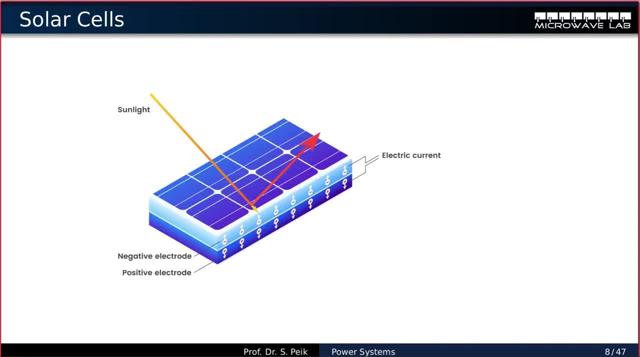 and the most enduring way to power up the satellite. Well, you're all familiar with how a solar cell works. There's sunlight incident into the solar cell and the solar cell has a negative and a positive electrode, So there's a p-n junction. 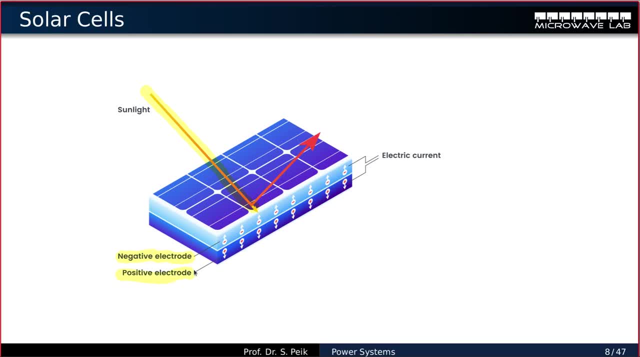 a semiconductor p-n junction, And from the physics of the p-n junction, the solar light is converted into a separation of charges. The negative charges go to the top, the positive charges go to the back. So And that way we create a voltage. 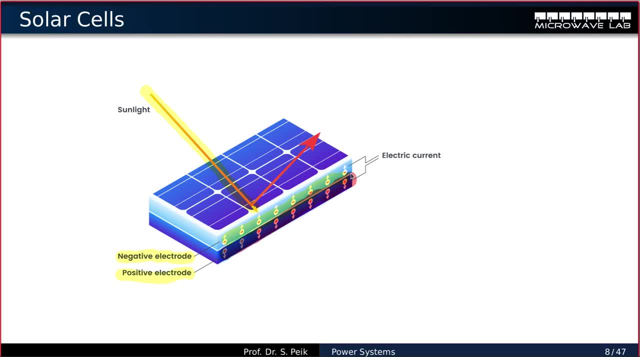 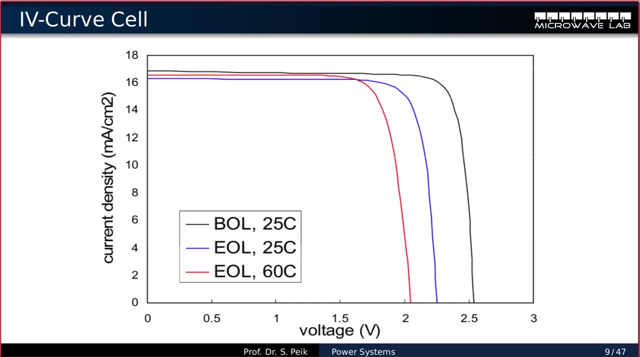 And when we put a load onto this voltage, we create an electric current and voltage times. current is my power that's generated by the solar cell. We can now plot the so-called I-V curve of a solar cell. That's the voltage observed on the solar cell. 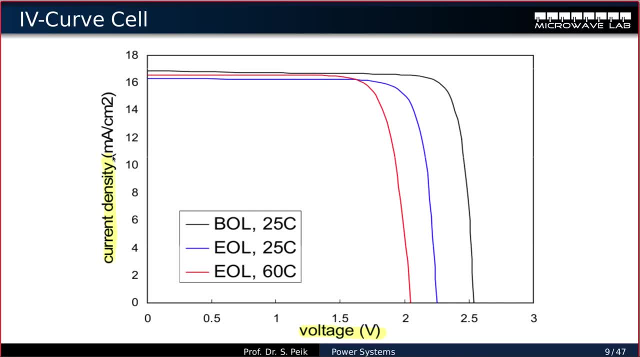 Depending on the load, we observe a current When there's absolutely no load on the solar cell. thelet's go here: the solar cell is open and maybe we can see a voltage of 2.5 volts, but no current, of course, because it's open. 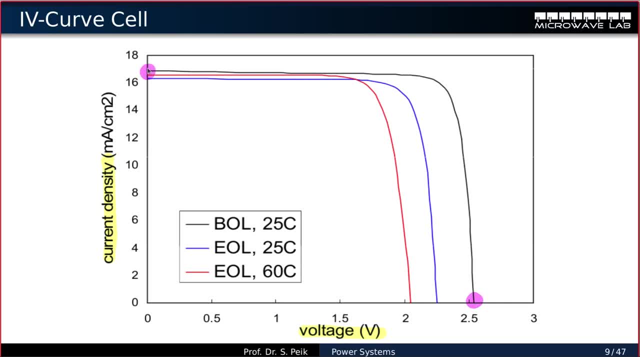 When we shore up the solar cell we get maybe 17 milliamps of current flowing but there's no voltage And, as you know, the power is voltage times current. That means either short or open is not a good condition And we have to go on that load curve of my solar cell. 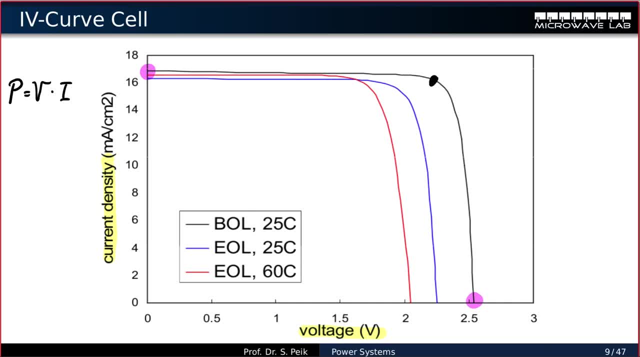 somewhere here At this point we get the maximum power out of the solar cell, because then we maximize our voltage to current My solar cell. that's shown here. let's say it's about 16 milliamps and maybewhat is it here? 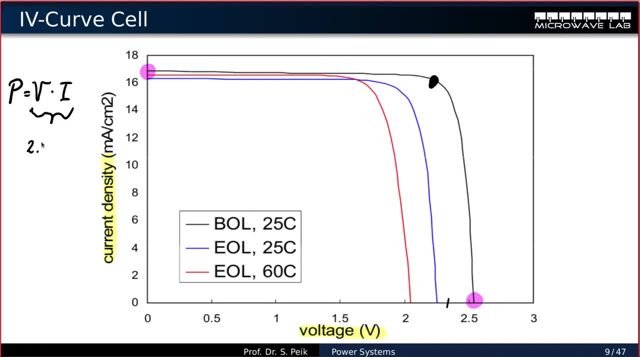 1.3 volts.2.3 volts. So it's 2.3 volts times 16 milliamps, And this is 0.038 watts, 368 watts. So that's my maximum power, Maximum power I can get out of this solar cell. 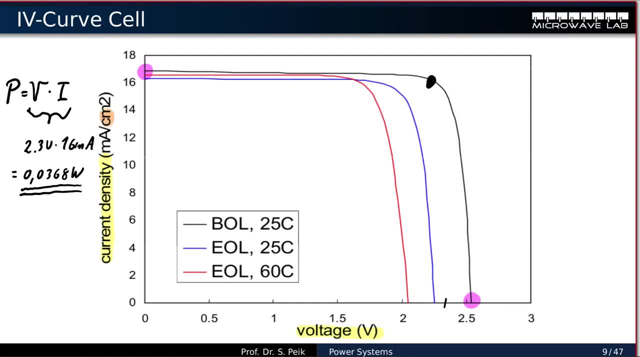 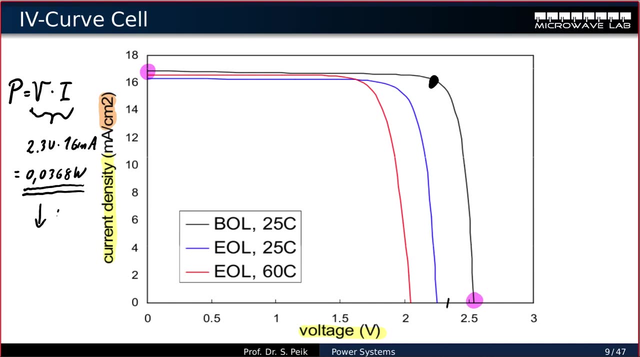 And note, this is per centimeter square, So one centimeter square generates 36 milliwatts of power. When scaling this to one square meter, that means I multiply this by 10,000, because per square meter, then I get. 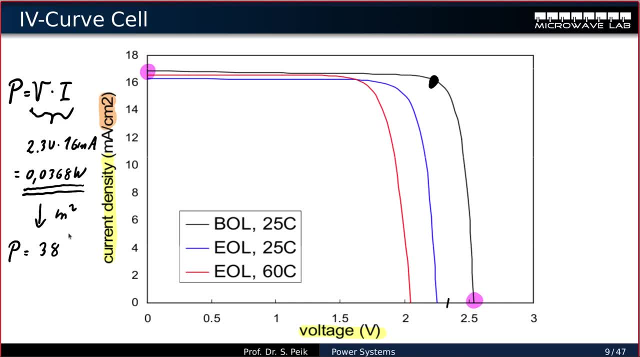 368 watts of power per square meter. And when dealing with a solar cell- and I don't have much space, maybe let's draw it here- Let's say: this is my solar cell. here There's sunlight incident onto the solar cell. 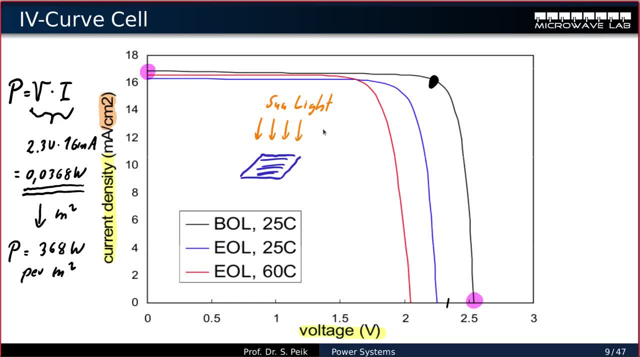 The sunlight has a power flux density, as we know from the antenna lessons, of a certain number And for solar sight in geo-orbit or in LEO orbit, it's about 1,370 watts per square meter. It's coming down on the ground of the Earth. 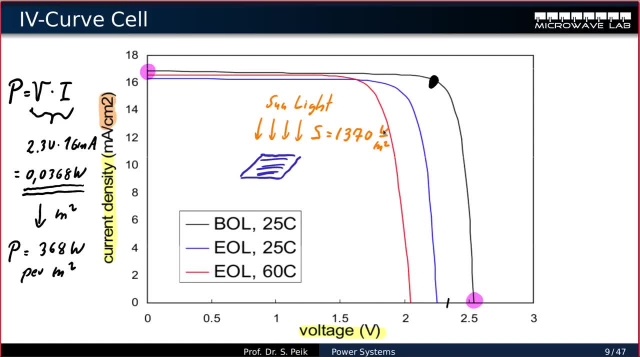 or in a low Earth orbit all the time from the Sun. So that means looking at it. we have an incident amount of power per square meter of 1,370 watts per square meter, But we get out of the solar cell we get 368 watts. 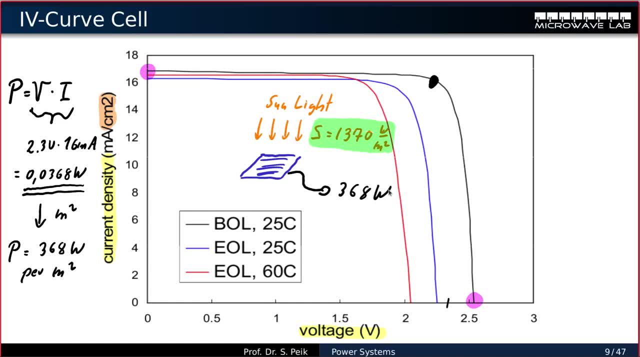 That means there's a considerable loss of energy from the Sun to the electrical power generated by the solar cell And this ratio is called the efficiency of the solar cell And the efficiency is my power generated per meter square over the flux coming in per meter square. 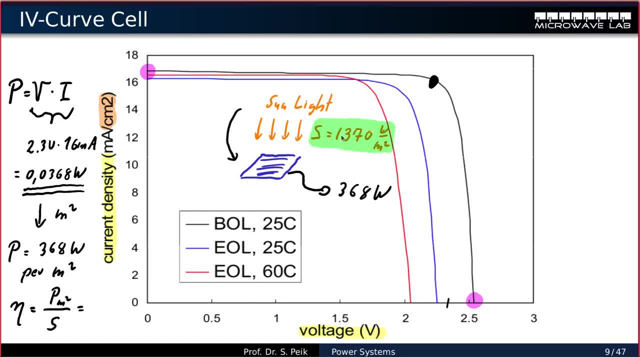 And when I'm dividing 368 by this number, I get, in my case, 26.8.. Now I'm running out of space here, so let's wipe this out. 26.8%, This is a fairly good solar cell already. 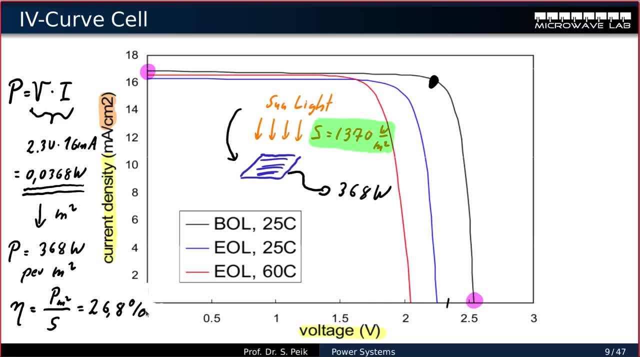 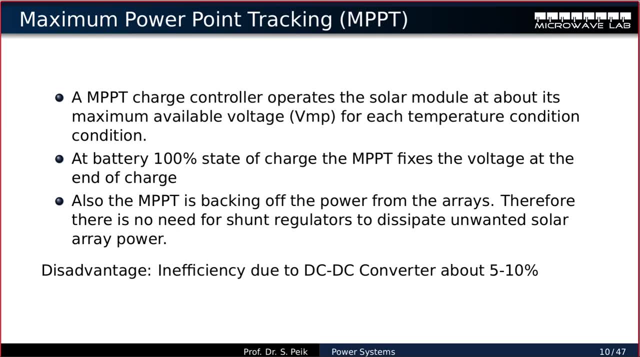 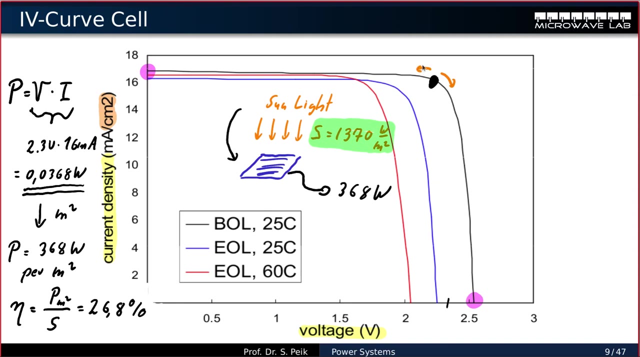 Typical solar cells have less efficiency than 26%. In order to get the most out of the solar cell, we have to use a so-called maximum power point tracker, MPPT. This MPPT does nothing else but moving that point around until it gets the most power out of the solar cell. 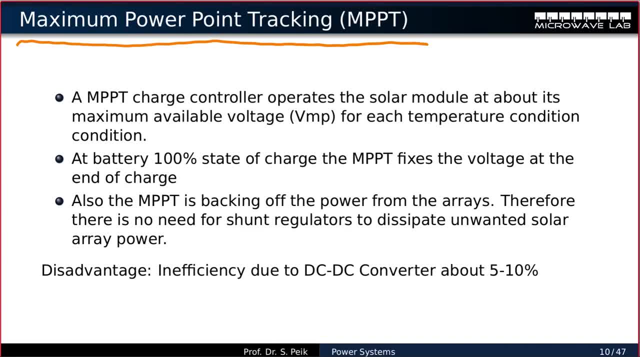 And it can also make sure that you have a certain voltage fixed if you don't have a non-regulated conversion. The disadvantage of a maximum power point tracking is well, the advantage is, of course, you get the maximum power out of it. 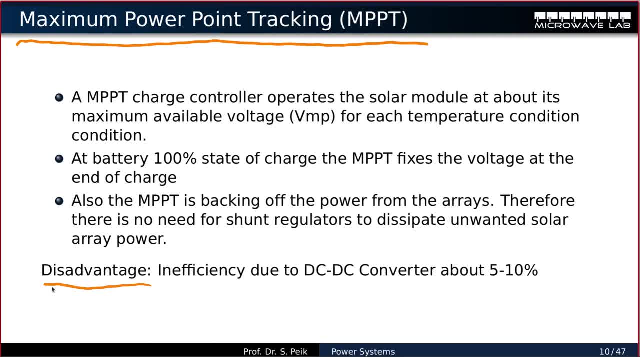 The disadvantage is you need DC-DC converters to convert from the optimum voltage here to the voltage you actually need for your bus, So DC-DC converters required. That gives you about 5 to 10% of losses again. However, you gain so much from the maximum power tracking. 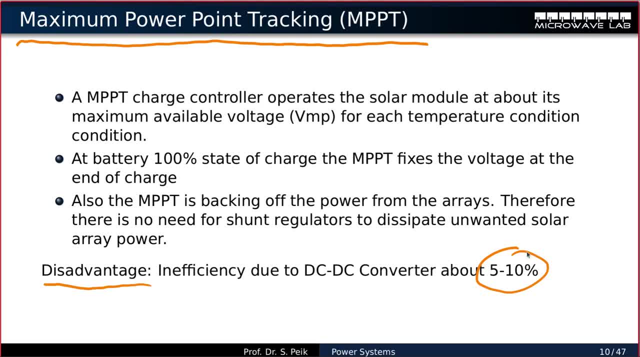 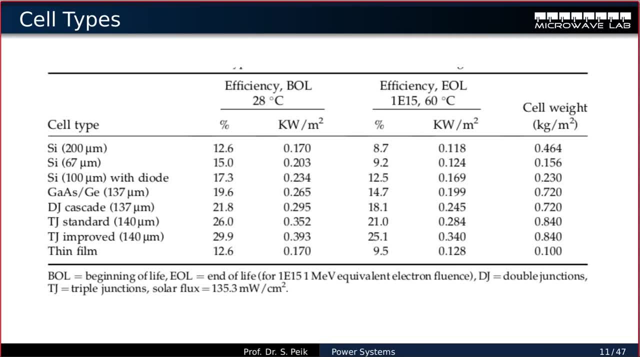 that this is usually acceptable. There are a lot of different solar cell types around and depending on the topology of the technology of your solar cell, you get quite a variation of efficiencies. Here's an interesting table of the efficiency of solar cells at the so-called begin of life. 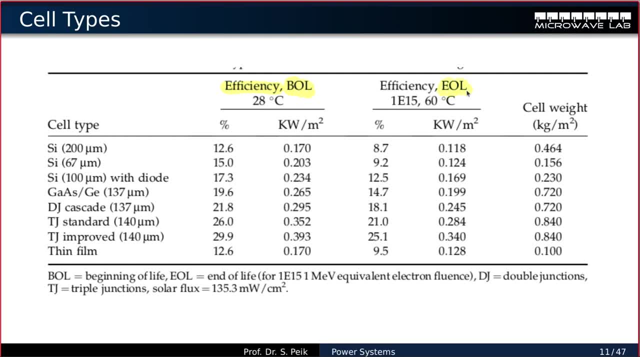 and at the end of life and after 15 years. That's here. I don't know why they call it E15, but I think they meant E. Oh, no, sorry, It's an electron flux that's coming in. 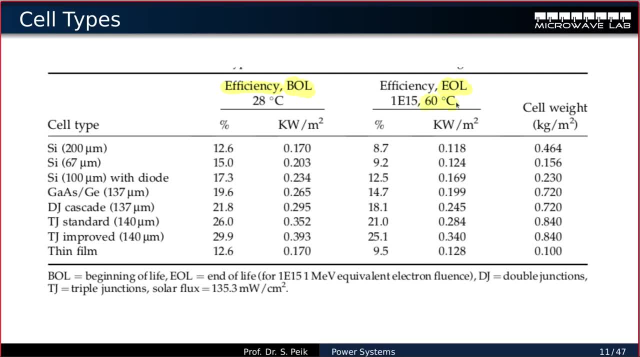 And also at 60 degrees. So basically, what you can say is: this is the worst case here And we always have to design for worst case. Now let's take a look. We have here the very simple ordinary silicon cell with layer thickness of 200 micrometers. 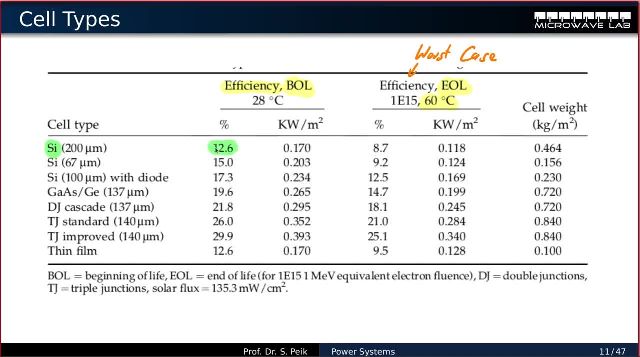 has an efficiency of 12.6%. These are the cells that are typically used in calculators and small appliances, which shall be powered without a power cord, And the advantage of those cells is they are very cheap, but the efficiency is fairly low. 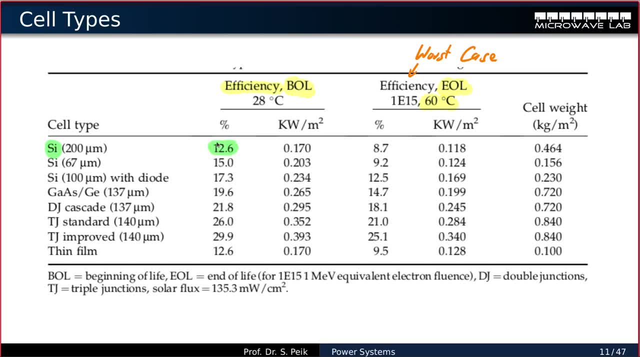 And when you do the calculations of efficiency times, incoming flux you get per square meters you get 0.17 kilowatts only At the end of life. the efficiency drops even to 8%, 8.7%, And also the weight is driver for satellites. 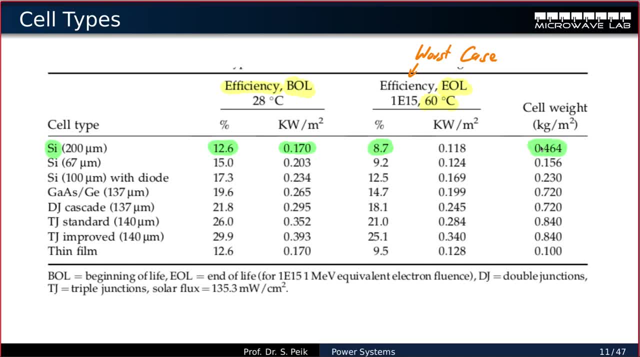 The weight of these satellites is very high because they are very thick And the so-called thick film cells. they weigh about 460 grams per square meter, which is quite heavy, as you see from the other cells. The other cells are better. 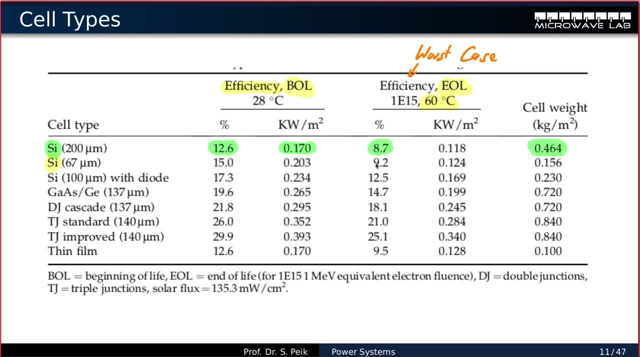 As you see here, the thin film silicon gets 15% or 9% at the end of life. Then you can have silicon with diets built in. They get a little bit more. And then very interesting are the so-called these gallium arsenide gas cells. 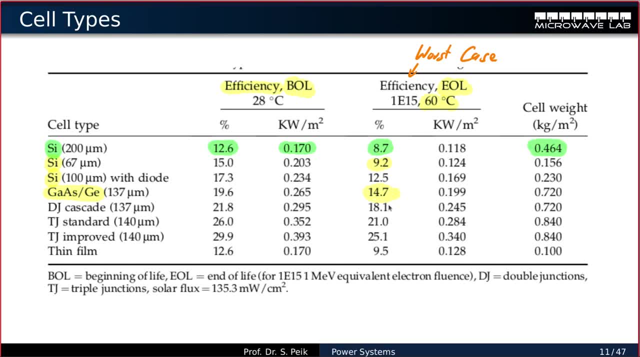 They have efficiencies of about 15%, And those are the cells that are often used for satellites, as they are a good compromise between reliability and heritage and efficiency. So the cost of the cell is not a major driver for satellites. You can pay more money for the cells. 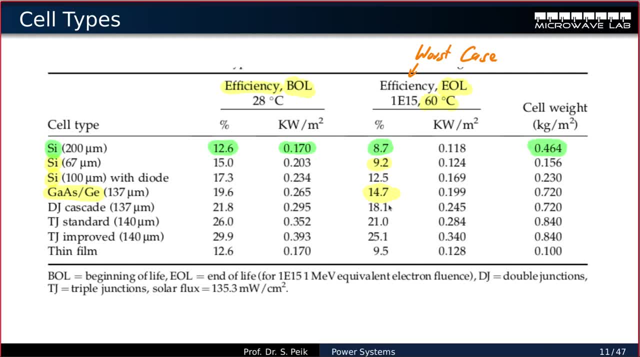 when you increase efficiency considerably and you reduce the weight. There are also so-called dual and triple junction cells. They are the state-of-the-art cells and they can get efficiencies up to 25-30%. So these are the cells also often used in satellites nowadays. 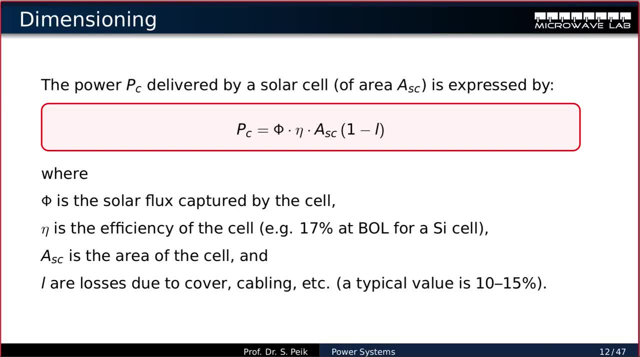 So let's do a little calculation On how much power you can get out of a cell. Well, it's now. it's actually quite straightforward because it's just a linear and logical relation between everything. So the power you get out of the cell is: 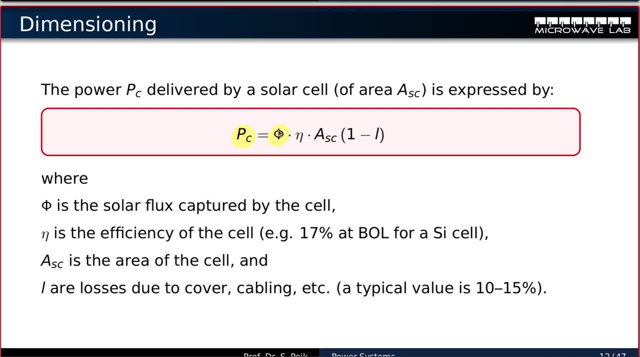 the incident: power onto the cell. That's the phi, That's the solar flux captured by the cell times. the efficiency we talked about on the last table times the area of one solar flux. That's the solar cell times, the losses included in the cell. 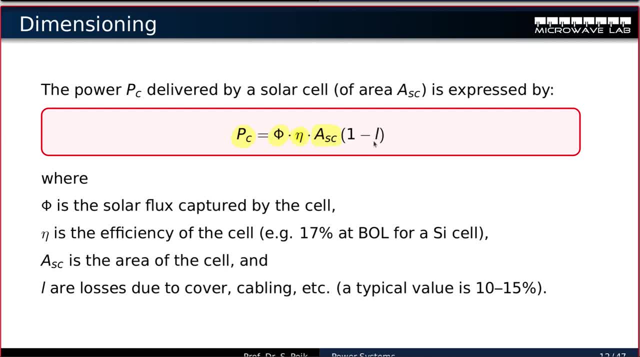 from cables and connectors and so on and glass covers here. So you have to reduce the 100% of the power by the amount of losses, So one minus L, And then you get the power that is generated by a single cell. What is my flux coming in? 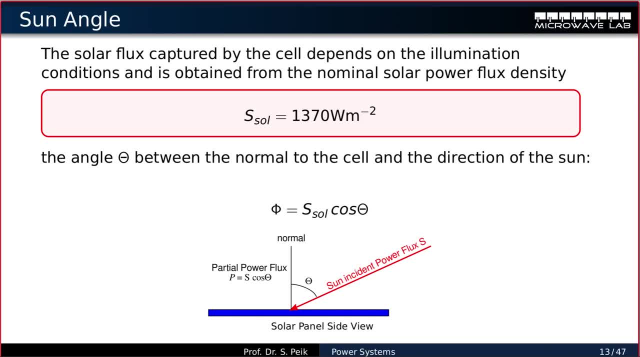 There are several things you can consider: The distance from the sun, the shading effects and so on. We leave those out for simplicity. We just say: well, we come in with 1370 watts per square meter. That's my incident power. 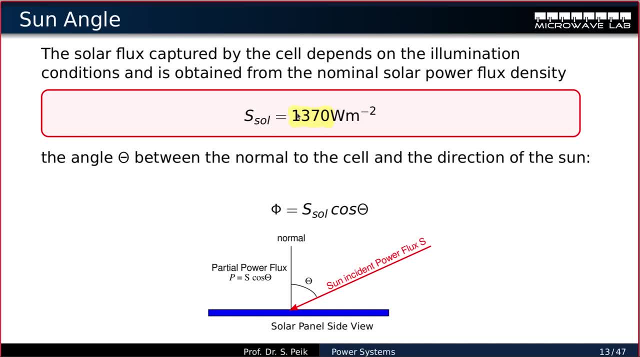 Some people use only 1350 or 1360, but roughly that's the value. It also depends on the solar activity and so on, But let's keep it simple. And then the incident flux is reduced by the angle of the incident power. 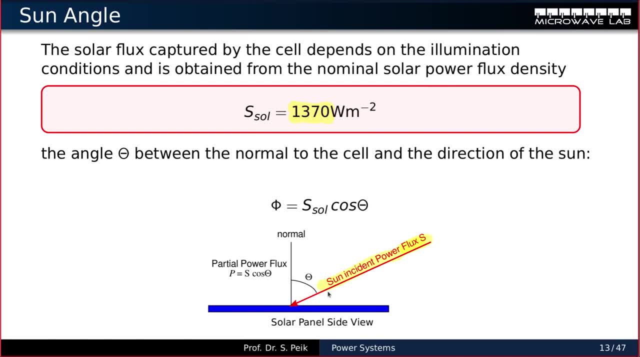 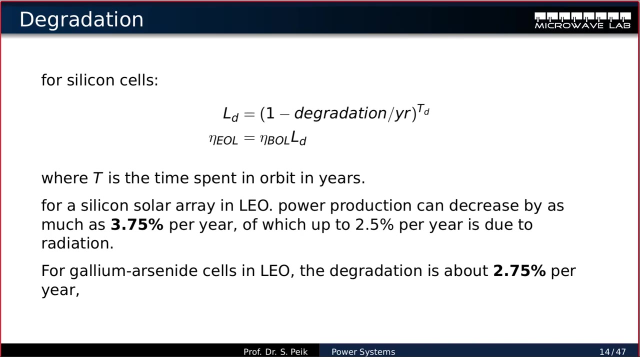 And obviously during trigonometry the incident power depends on the angle by the cosine. Normal incident means 100% of the flux, 90 degrees means nothing And in between we have this cosine relation of the flux. We also have to put the degradation. 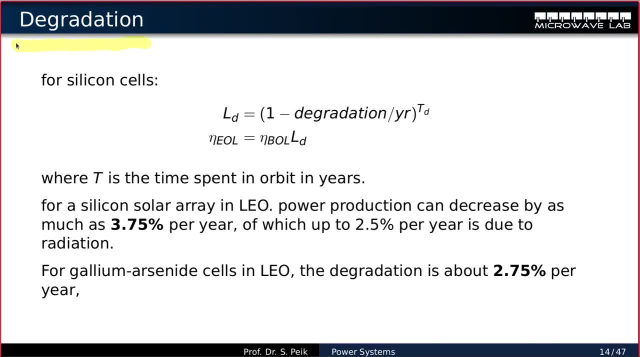 of the cells into consideration. As I said, over time the solar cell degrades because it's bombarded by electrons and other ions in the vacuum space And that reduces the efficiency of the cell And the efficiency at the end of life is reduced by certain factor, LD. 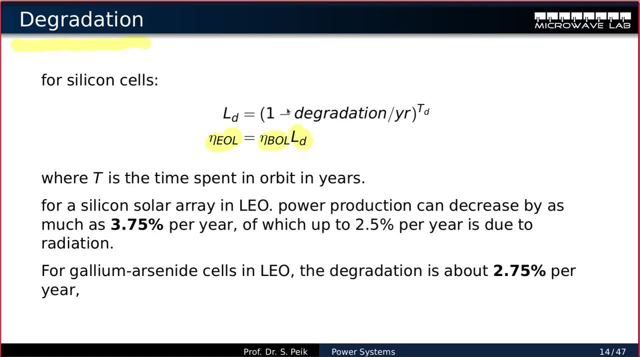 Which is exponential decay, one minus degradation per year. And typically you have for silicon cells about 3.7% degradation per year And the gallium arsenide you have maybe about 2.75% of degradation. And then when you plot that, 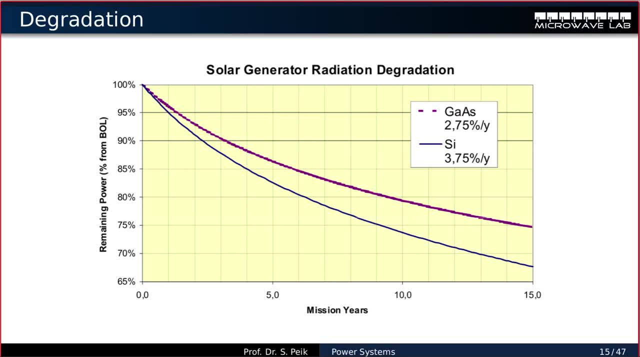 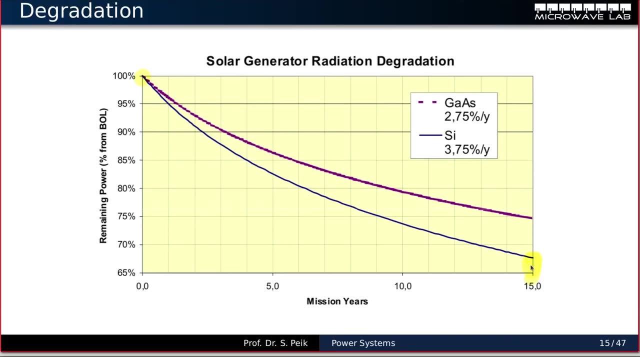 it looks something like this: It depends on how you do your compound interest formula. You start with 100% of your begin of life and then at the end you end up. after 15 years you end up at maybe 65-60%. 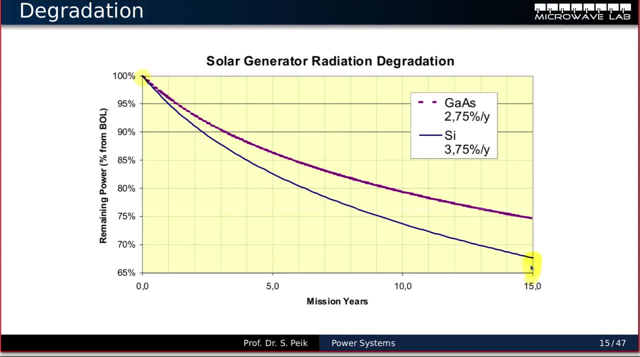 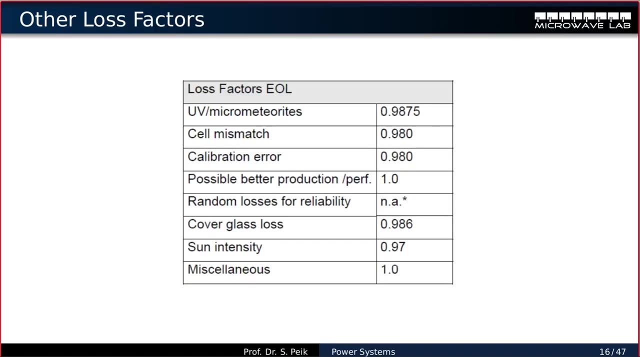 of your initial efficiency of the solar cell. That means after 15 years you can usually say: well, we go towards the end of the life of a solar cell and we should consider giving up the satellite at this point. The other loss factors: 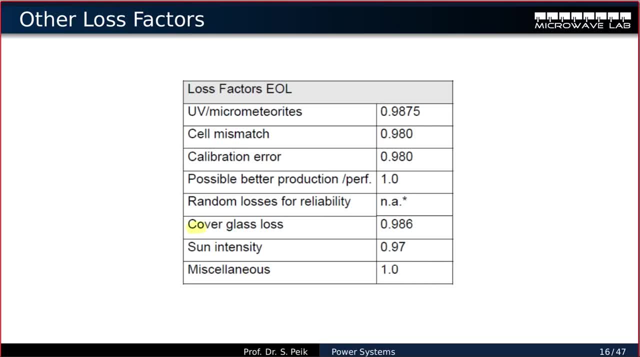 I don't want to go through all of them here, but for example, when you have a glass cover that reduces the light a little bit, the sun intensity varies over the year and over the sun activity You get mismatch between the cells, and so on and so on. 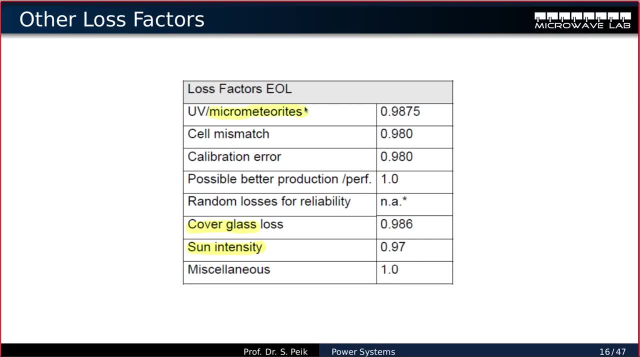 And you get micrometeorites hitting the solar cells. They are dust particles basically destroying part of the cells, And things like this reduce the efficiency and maybe when you put it all together- oops, when you put it all together- maybe you get another 5% loss. 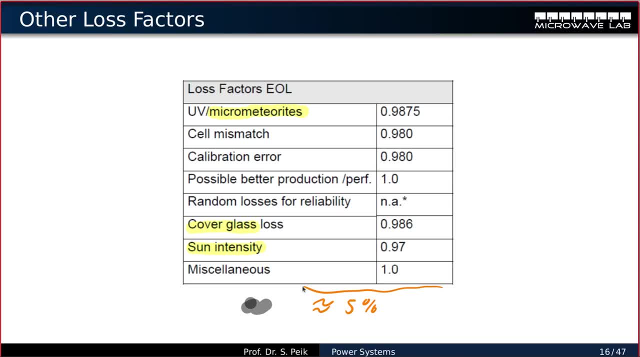 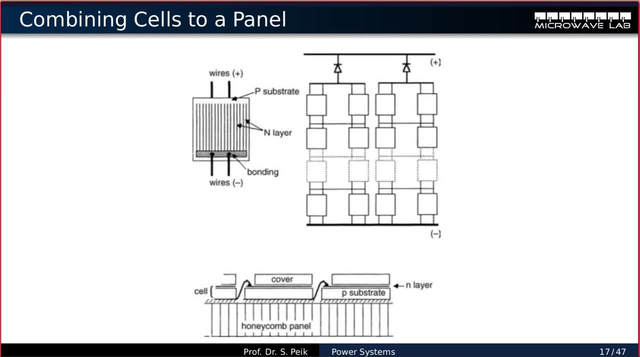 from all these things put together, One cell is good. Many cells are better And as an electrical engineer that shouldn't be a problem for you guys. When you put here, let's say, four cells in a row, then the voltages of the 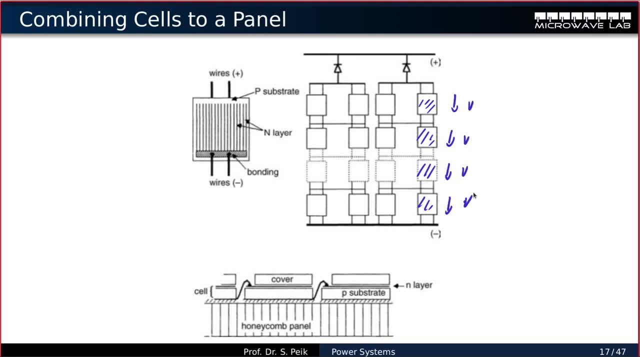 of the cells add up. That's a simple way of increasing the voltage of the cells When you put them in parallel. the currents add up The currents, basically. So typically you put diets in the, in the rows of the cells, And you do that because 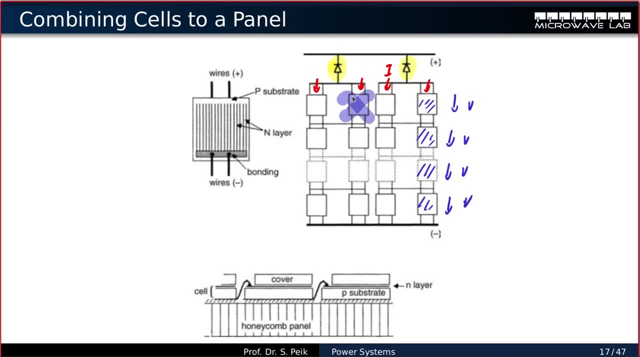 if there's a solar cell failure, for example here, then if the solar cell doesn't produce power anymore but it consumes power, and that would mean that when this cell row generates power, it will go as a consumer into this cell row. 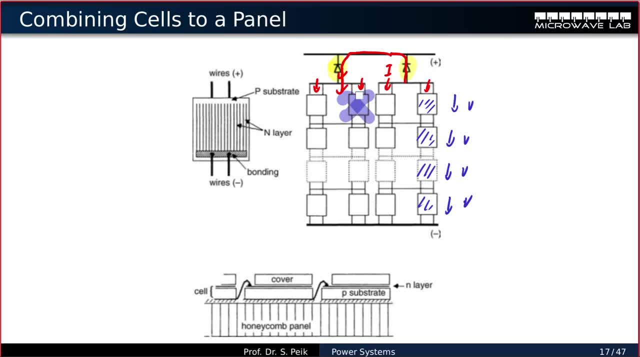 And in order to avoid that, you put the diets in there And you don't have that problem. Okay, That way you put them together. The solar cells are little glass plates And in order to make a panel, you put it on a honeycomb panel. 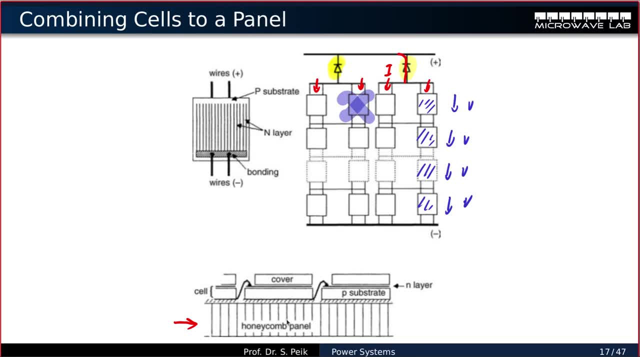 That's a very lightweight plate, basically, And then you put them in a row- Here this is a solar cell- And then you put a cable from cell to cell And that way you can put them into series And then, typically, 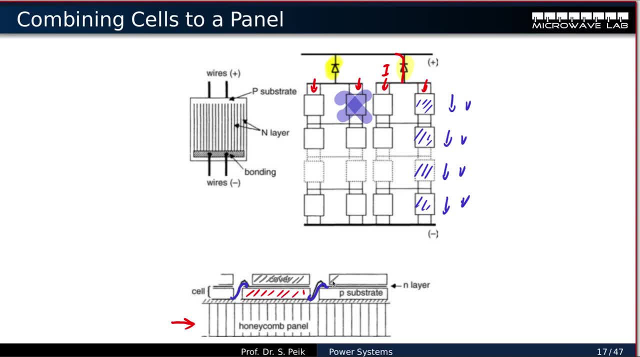 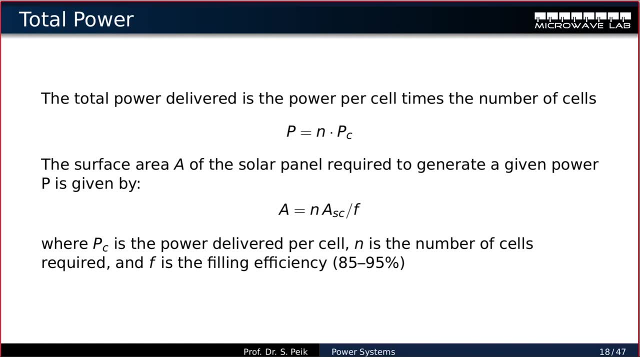 you have a glass cover here to protect the cells a little bit from the outside world. So now my total power is now the power delivered by one cell times. the number of cells is the total power, obviously, And the total area you need. 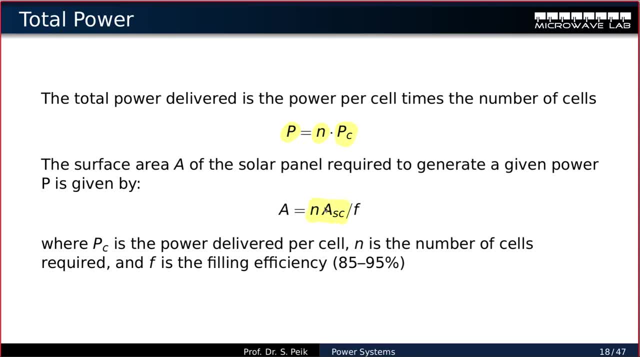 that's covered by the panel is the area covered by one cell. here times the number of cells, And then you also get the so-called filling factor, because not 100% of your area can be filled with solar cells. You have cables in between. 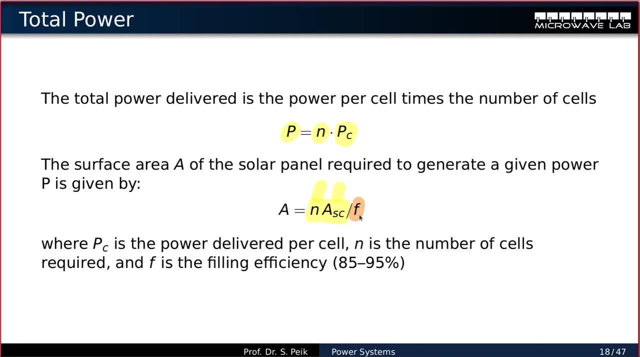 you have contacts, you have glue and so on. That means you lose some area, And that's typically about 90% of your area is only filled with solar cells. The rest is cabling And having all these equations, we can now 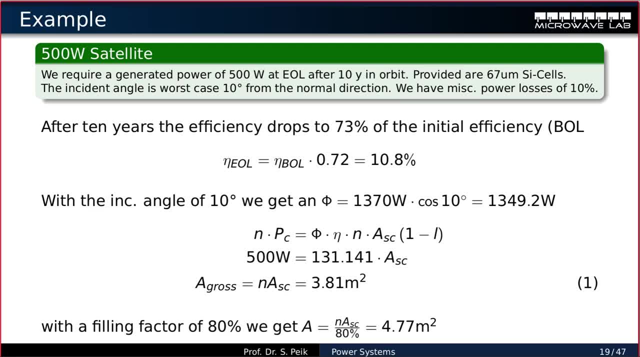 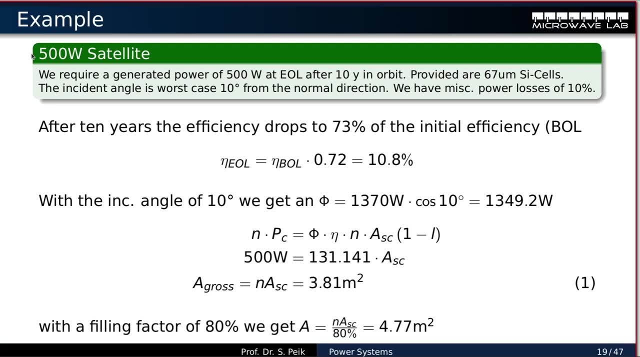 calculate a typical solar panel In my example here. let's say we have a satellite that's supposed to provide 500 watts And it should be 10 years in orbit, and we use 67 micrometer cells and my incident angle is 10%. 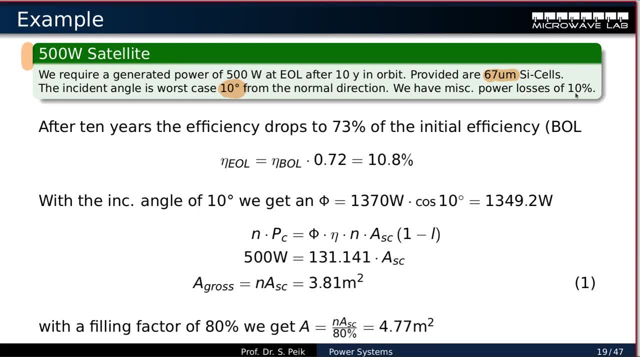 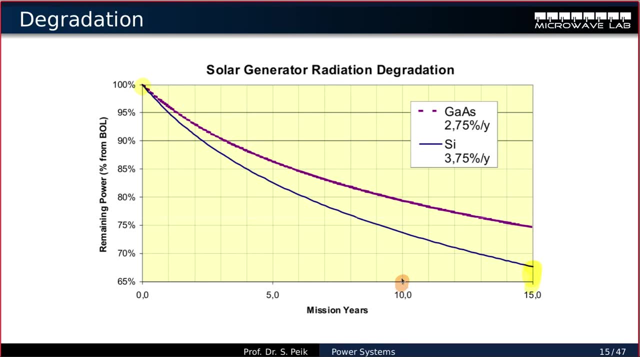 from the normal direction And we have also power losses of about 10% miscellaneous. Then we can calculate our efficiency drop from- I just used my graph here- this here- silicon cell. so we are here. that's 73, 72%. 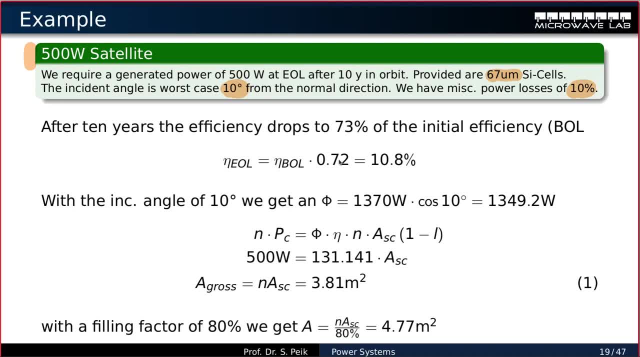 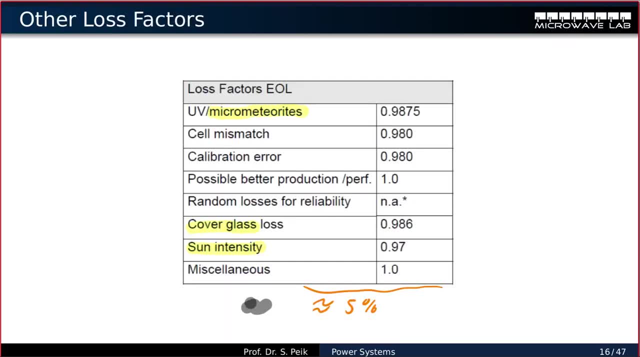 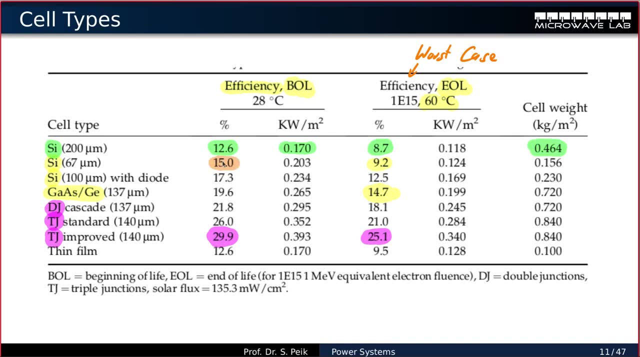 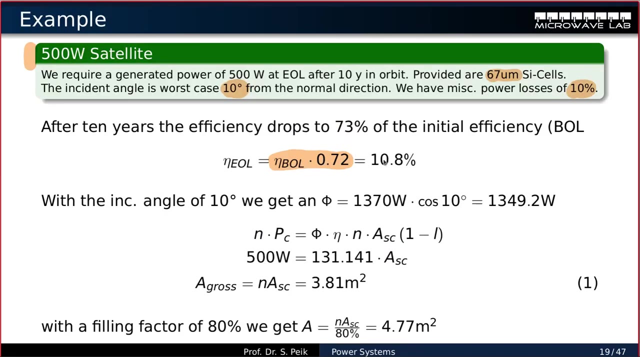 That means at the end of life. my begin of life is only 72%. Begin of life. let's go back. Begin of life. we are here at 15%. That means times 0.72, we end up with 10.8%. 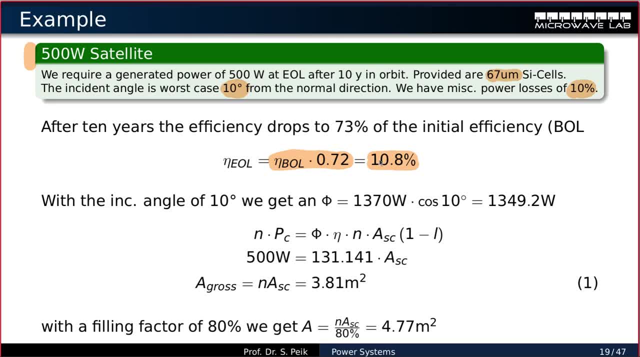 Okay, good, So that's my end of life efficiency. Now. our incoming flux, Here, phi, is the 1370 watts of solar flux times. cosine 10 degrees gives me 1349 watts of incident power, And now we can calculate the amount of. 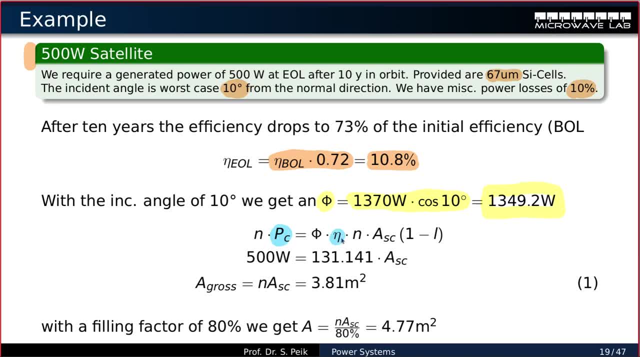 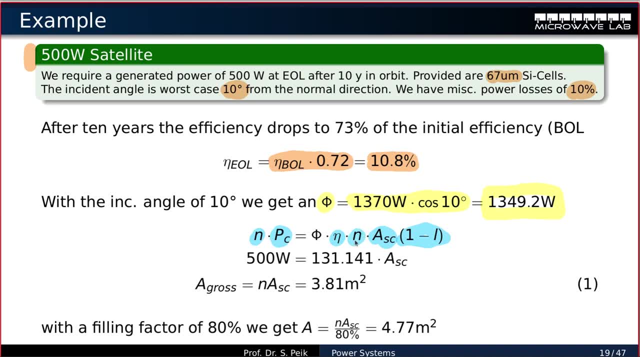 power by this. So that gives me the cell which is my efficiency times, my area times, my losses, And then we multiply it by the number of cells And that gives me my relation between the total power to the power by cell times n, and so on. 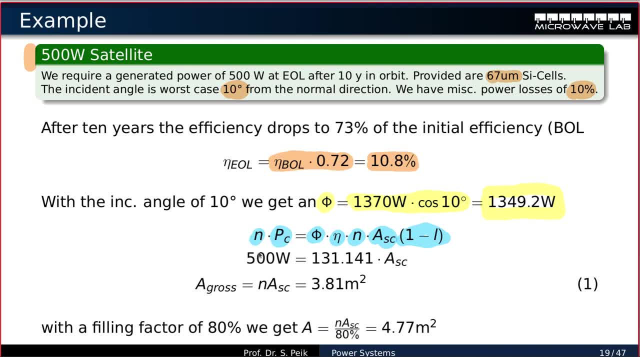 Since we know the left side should be 500 watts, we can put together all the other things and we get an area of solar cells, which is actually n times, which is a number we can calculate, And then we get a solar cell area. 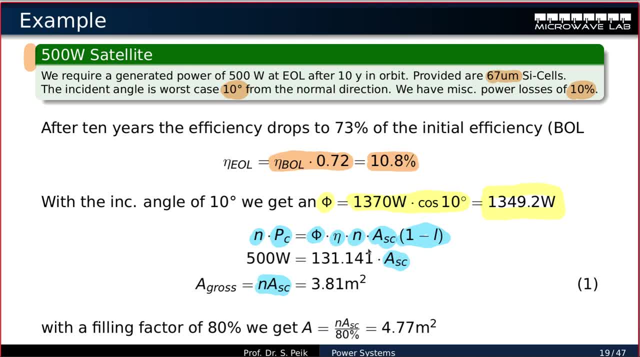 of n times my SC, So the n is. I missed the n here. no, that must be times n. n times SC becomes, doing the calculation, 3.81 meters squared. That's my gross area, Since we have our filling factor. 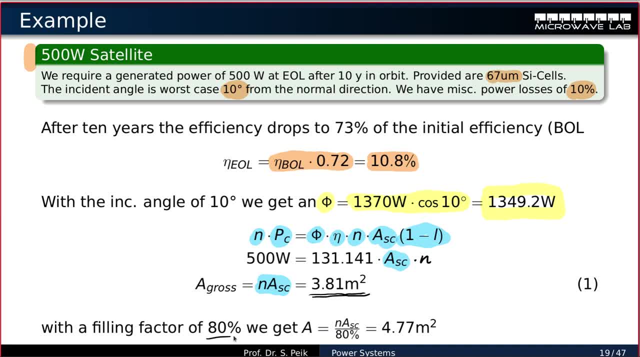 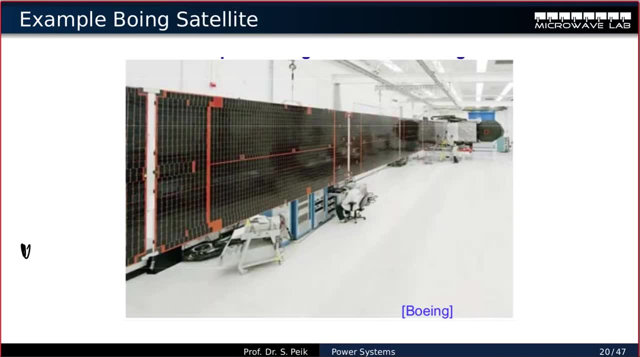 of 80%. well, I just assumed this. here I need a total area of 4.77 meters squared of solar area, solar cell area as a panel. So, as you see, these panels can become very large. This is a human here. 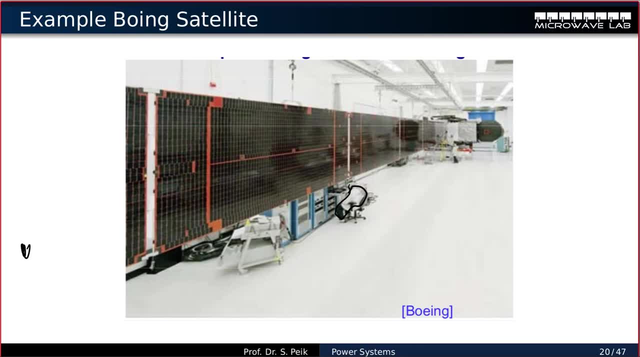 not this guy, Oops. So this is a person And you see there's a fairly large area. This is a TV satellite And TV satellites need a lot of power because they distribute the power on a large area on the ground, And that means 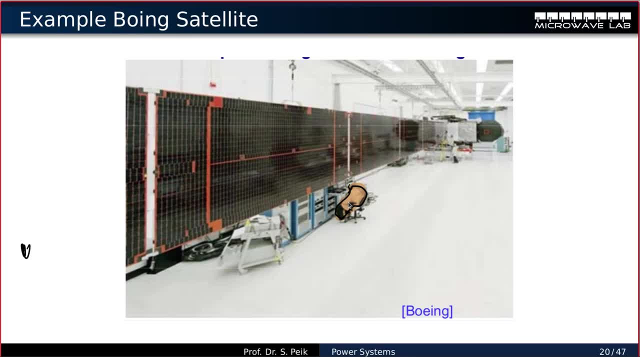 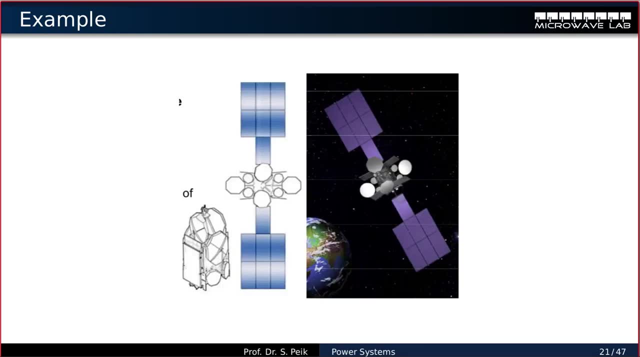 you need thousands of watts and you have a very large solar cell area here. The solar cells are a problem during the launch because they are very large And you have to fold them together. And here you see one example. I forgot which satellite it is. 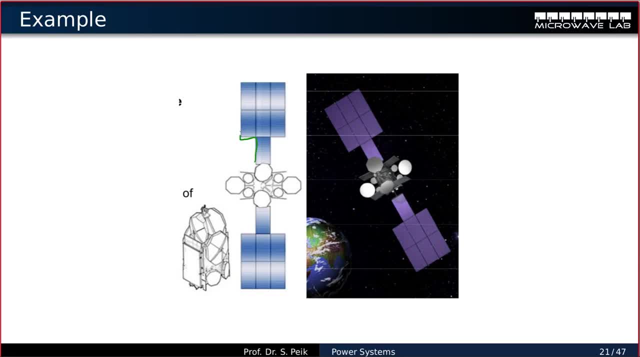 which shows how the solar cells in space they are unfolded like this, And then you have to do this origami kind of thing to fold them together. so the solar cells go as a package around the satellite And usually they are spring-loaded. 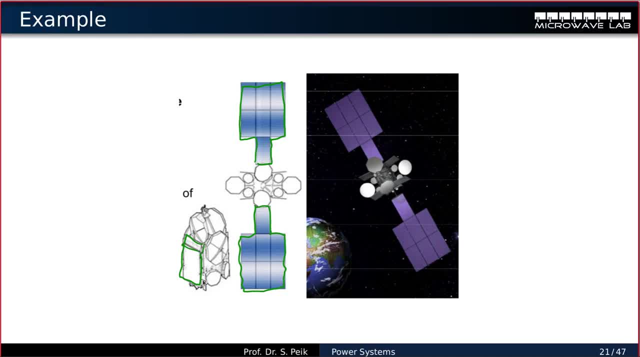 Once they are in space, they have this little screw. You open it up and from the ground command and then the solar cells unfold. This is a very critical moment of the satellite launch. If this unfolding doesn't work because something is stuck, 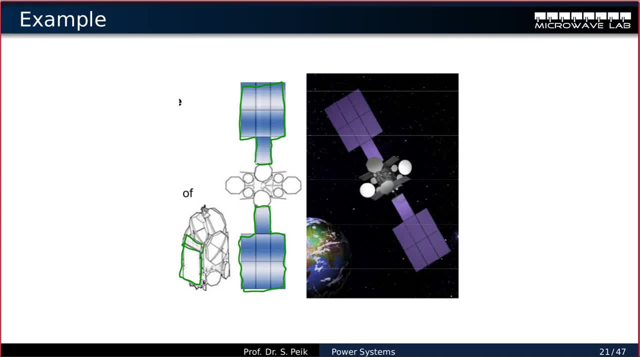 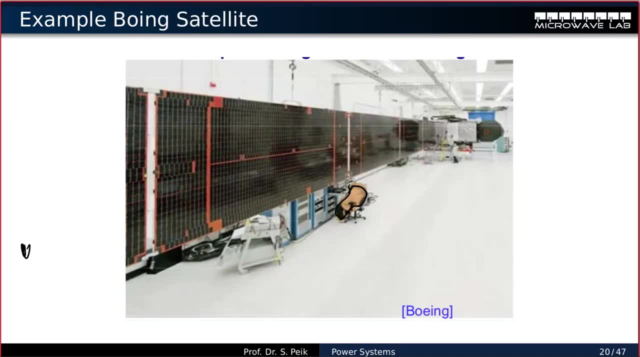 then, basically, the satellite is lost because you cannot generate the power you need. That's why you have to make sure that the unfolding mechanism works, And that's not easy to test on the ground, because on the ground you have gravity and in space you don't. 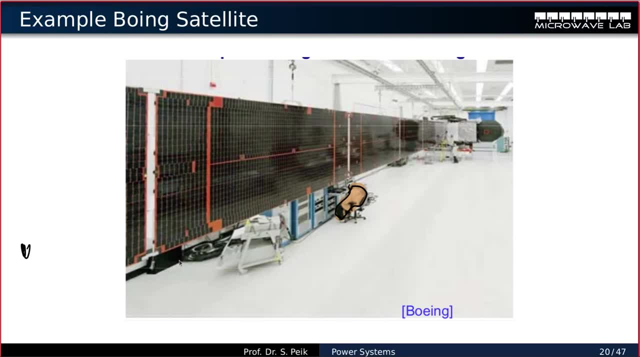 So this panel is hanging down to the ground from the gravity, and in space it doesn't. That's why they have here, you see, these little cables. They hold them up with cables to compensate the effect of the gravity on the ground, to see how it unfolds. 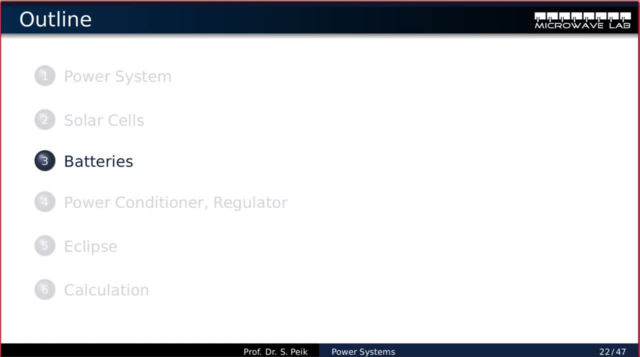 Okay, this concludes the part on the solar cells and we continue with the batteries.